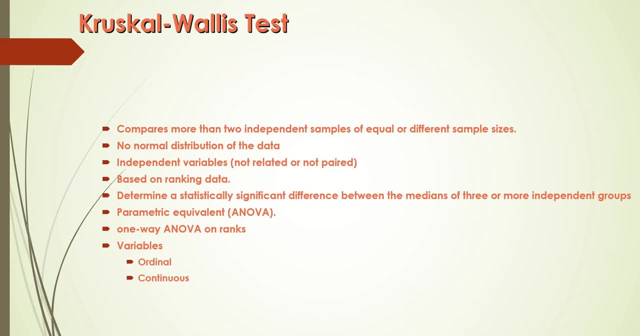 distributed in one of the group or in more than one group doesn't have a normal distribution that delete the groups. variable within the groups are independent. they are not related, not paired. the test is based on ranking data. the test determines a statistic, a statistically significant difference between the medians of three or more independent groups. so it is specifically 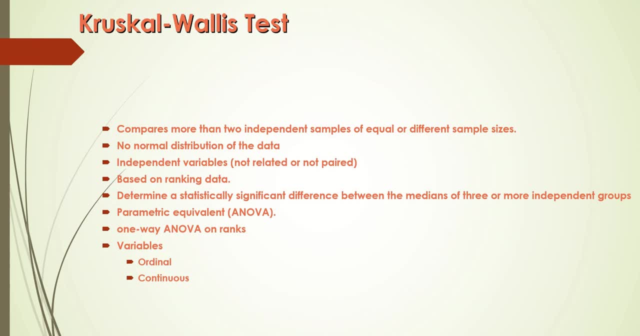 designed for a set of data in which you have more than two groups, three and more. the test is a parametric- parametric equivalent of ANOVA. it is a one-way ANOVA on ranks and the variables within each groups either can be ordinal, an ordinal. 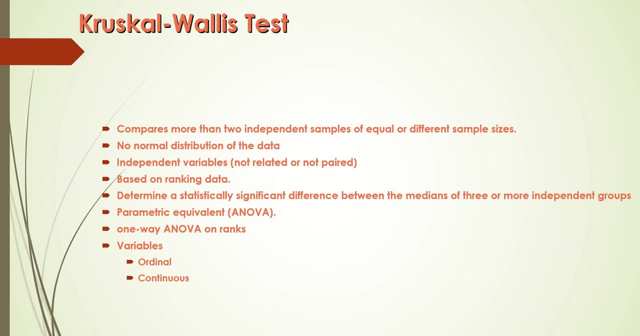 as I has mentioned before in different video clips, ordinal is from. a number is five, one, two, three, four, five, one mean unsatisfied, five, mostly satisfied or mostly agreed, or the variable can be continuous, in continuous, like weights, height and so on, but the data on this in this continuous variable is not normally distributed. 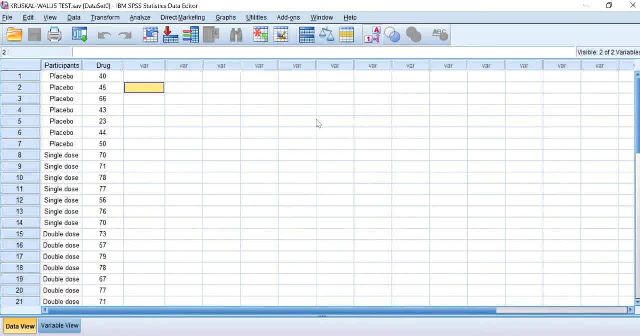 so how to do the analysis if we go into the spss window, in data window i have generated really here at the result, or data in which i've within, in which in the in this data, i had really 21 participants in a study in which a new drug has been produced and then need to test the efficacy. 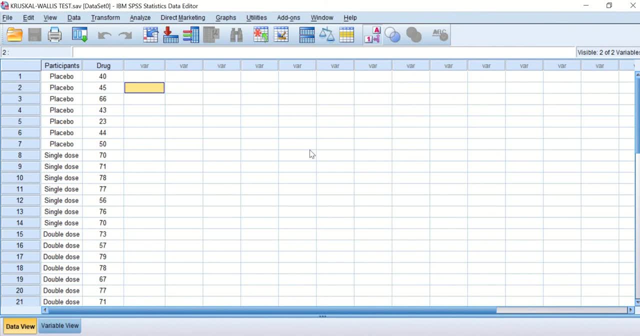 and effect of this drug on one of the variable in effect, on one of the variable in effect on the blood component, the efficacy of it. so this group has been divided into three. the first group has been given a placebo, which is really not a drug, anything like water. 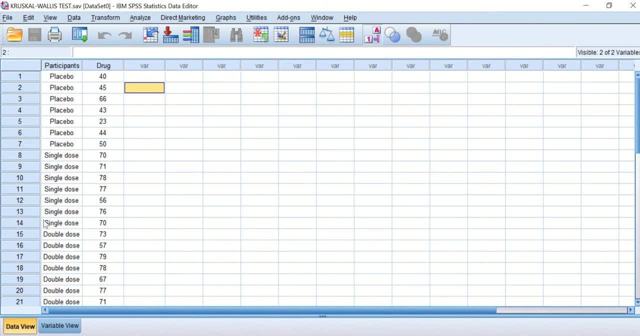 or salt and so on. the second group just giving single dose of the drug. the third group given a double dose of the drug. and then the drug efficacy was measured, as we have seen here, through a number, given a number which means that the drug had a more effective effect. so just see here the 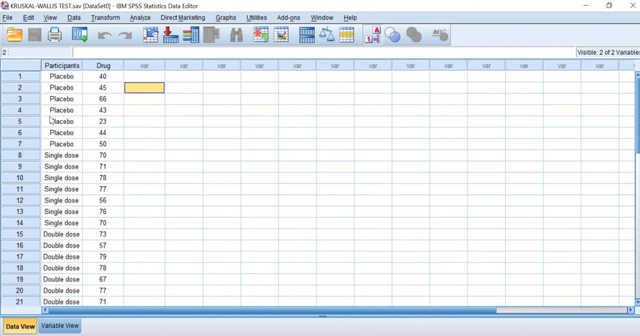 so, as we can see here, the group size is small. all the groups are seven. in each group there's seven participants, and I've checked the distribution of the data in the drug section, or variable, and it was not normally distributed. so how can we really calculate? how can we calculate the significance of the drug? 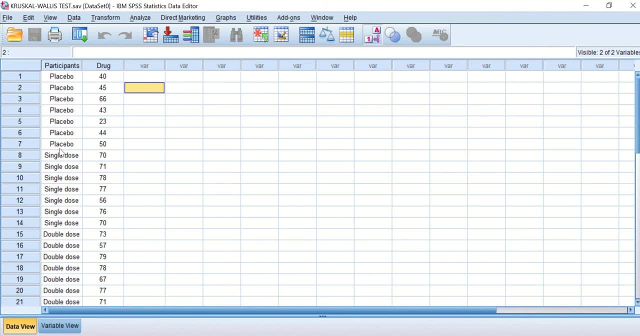 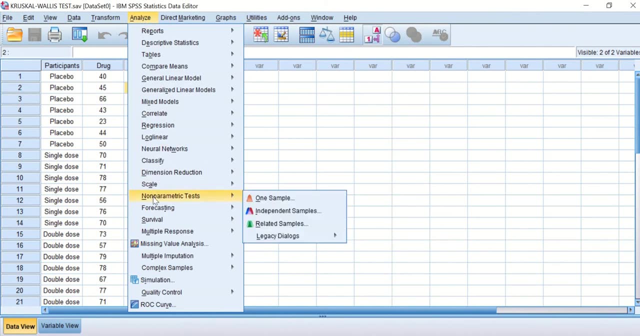 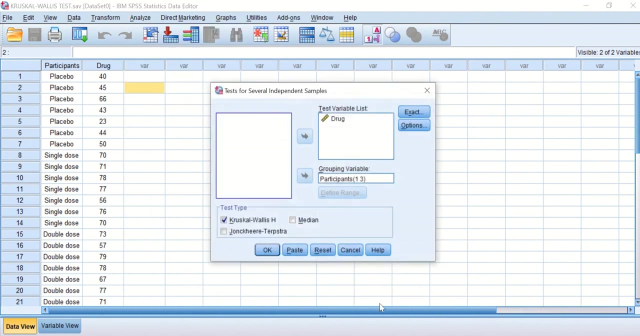 between these groups. okay, the way to do it is to click on analyze, scroll down to non-parametric test, because this is non-parametric data, and then click on legacy. then scroll down to K- independent K, indicate that more than two samples, click on that and then reset that. another window will appear in that. 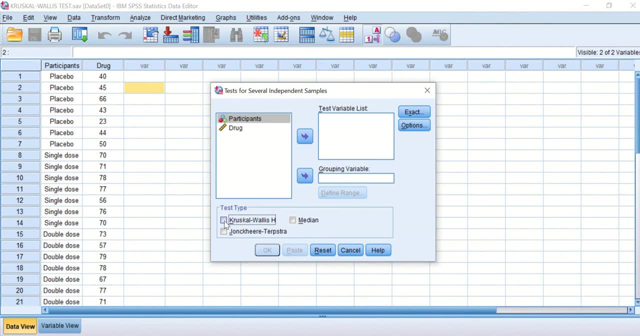 window. there is a test type called care scale will click on that. so we need the cash cow cascades well, as test with trot transfer. transfer a drug into the variable list to test the variable participant. we will move it into the group variable and in the group variable I'm going to tell the software. hey, listen, I want you to look. 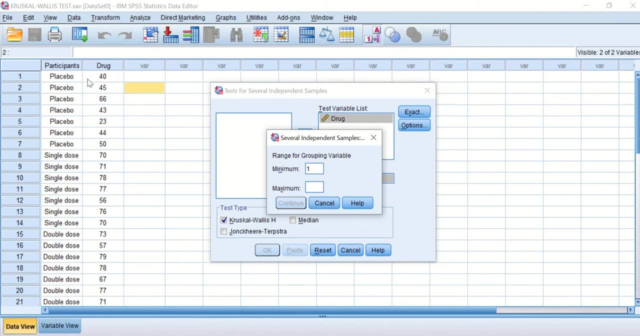 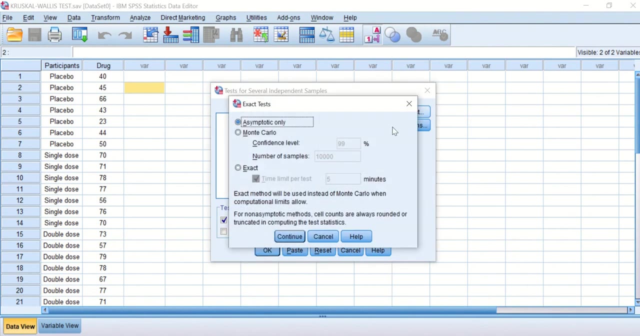 at the group from number one number. when I give it, it has been assigned for placebo to maximum number three. three is uh, from one to three. so the placebo single dose and double dose and then click on okay, continue for the exact link. look in the exact test. we'll just give it a same symptom to take. 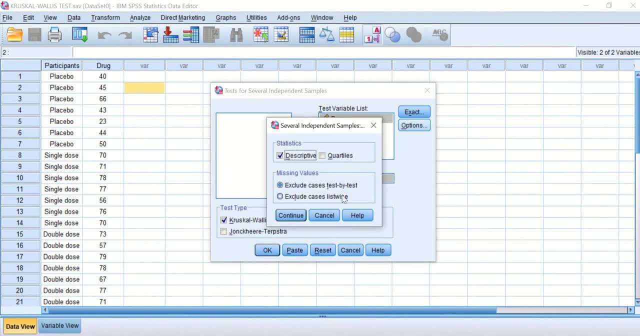 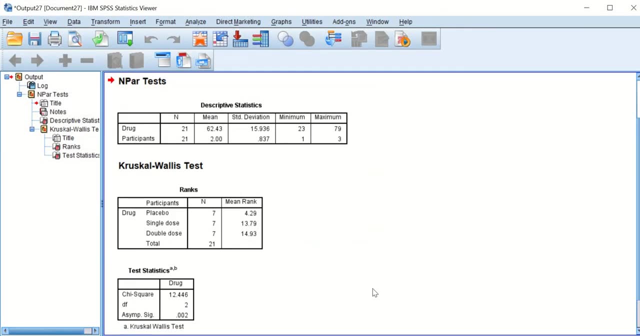 only, and then the options. i will select descriptive and then i will click on continue, then hit the button for uh, okay, and then uh, an output spss window will appear telling you the drugs has been part. there are 21 part participant on this study. it will calculate the mean and the. 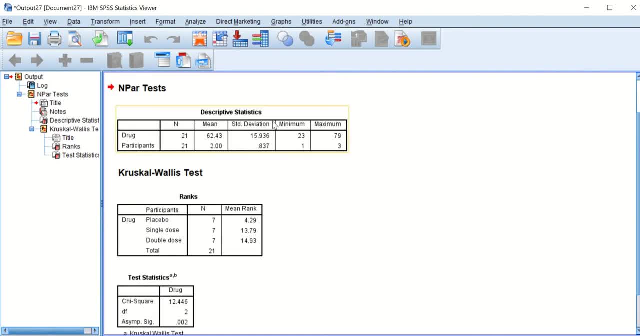 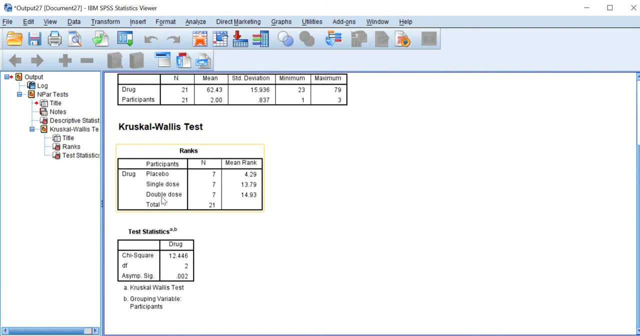 standard deviation. however, what's important as this is, descriptive data wall occurs- cal wallace test. as we can see here, three grooves: placebo, single dose, double dose and, again, as you can see, there are seven participant individuals in each group and if we look at the again, the care scale ignored the value of each uh number in the drug and rank them. 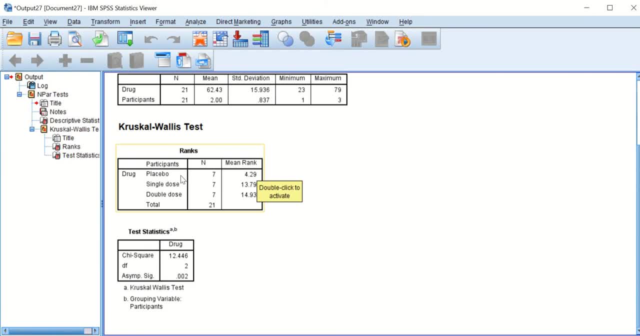 didn't work in the actual data. it took the these data and rank them and put them in rank and give it a rank. so the mean frank for the placebo is 4.2 and for single dose 13 and for double doses 14.93. as we can see, there is a difference in the mean between placebo and single dose placebo. 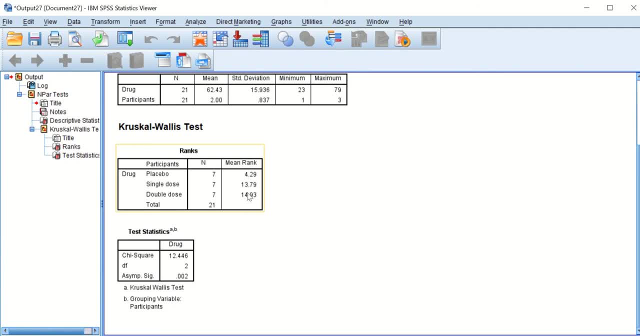 and double dose, but there is no seeing no difference, not significant, not that much difference, let's say, between single dose and double dose. now kerskal wallace tests in spss has calculated the overall significance and comparison between these three groups and found out that there is a significant differences between these. 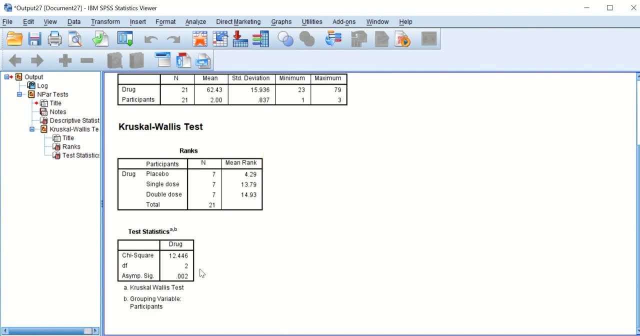 groups- ie taking the drugs- make changes, but doesn't specify which two groups are significant and which are not significant. as we can see here, the mean rank between single dose and double dose is very close. so if I want to find out which groups really giving a different has a significant difference specifically, 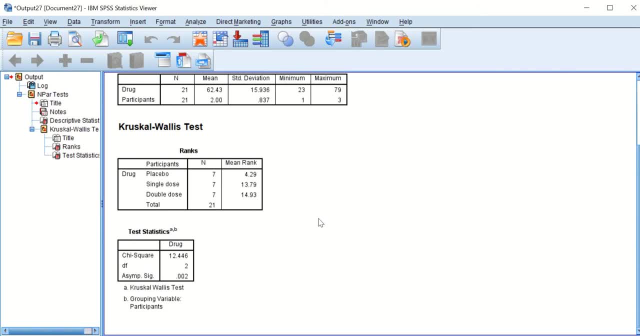 significant difference or effect of the drug. we need again instead, in addition to do care scale, to go back again and do man with new test for placebo and single dose. placebo and double dose, then single dose and double dose, and I will show you really how to do it. I've already shown you how to use man with. 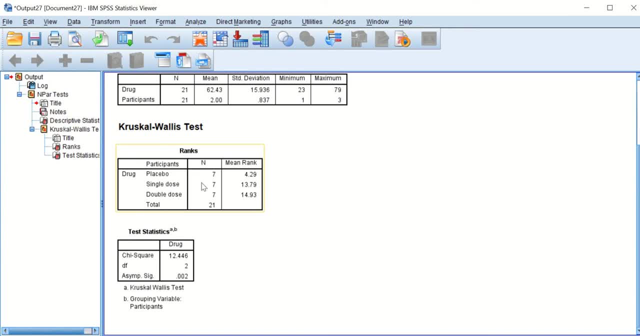 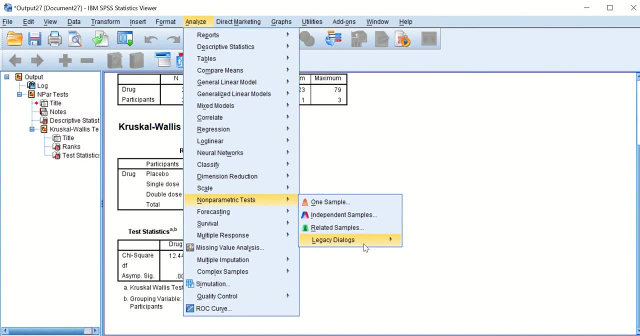 new test in a previous video clip. you can have a look at it. but the way to do it is to go analyze, click on non-parametric again and then click on legacy dialogue and then we need to click on two independent, because these data we have our independent, so we click on that. 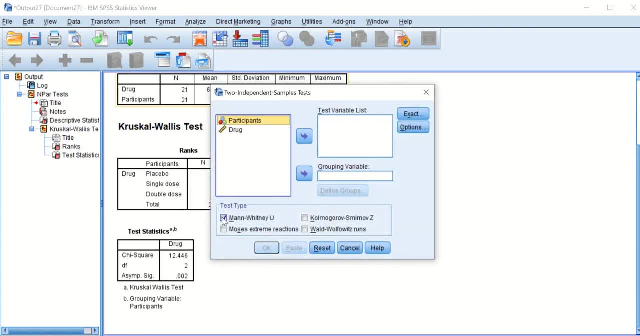 reset that again, again and I need to click here on man with new test. I need to put the drug in the testing one and the participant here and I will come. and then I want to define the group. here we need to test, compare, test to group together. so group number one is the placebo type one and a group number two. 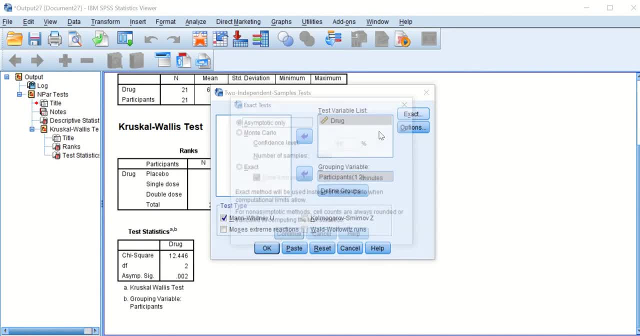 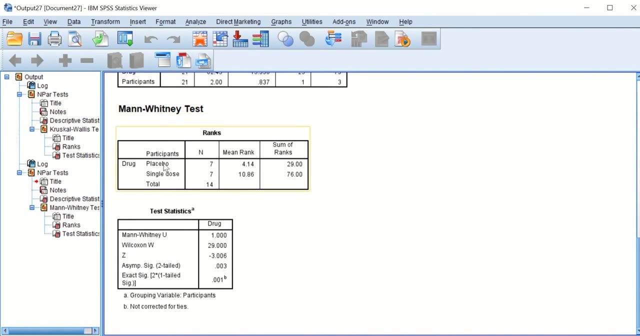 is the first single dose. click on continue. exactly, we'll leave this. this i window is exactly the same for option. we'll take only click on descriptive and then we'll click on continue, hit the okay bottom and voila. we see here that the man with new test has been calculated for placebo and 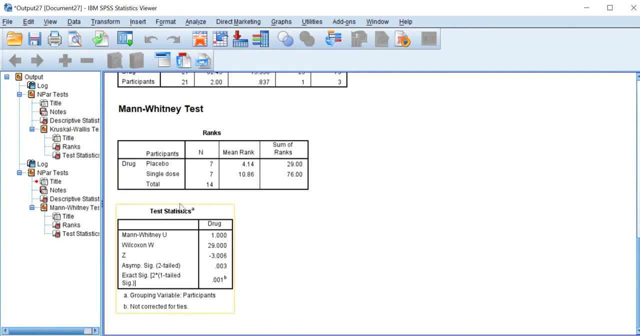 single DOS and it was found that there is a significant difference, that if you get the phase dose of the drug, you get really a difference between control- you, which is a control, and the single dose. so there is a significant difference. now let's see if there is a significant difference between a placebo and a 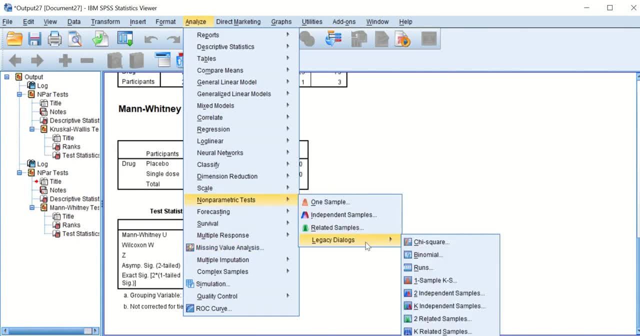 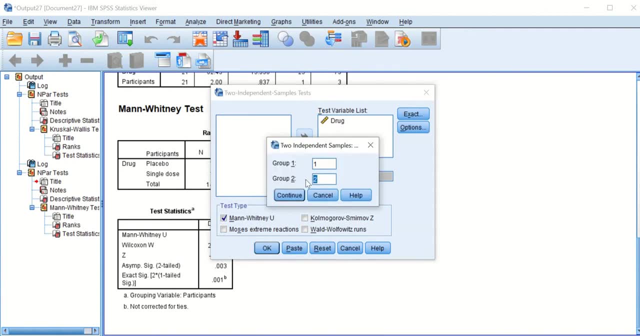 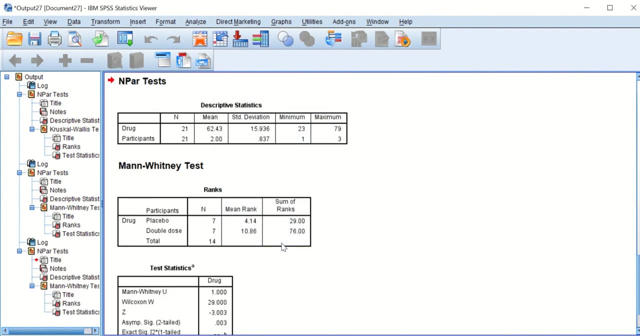 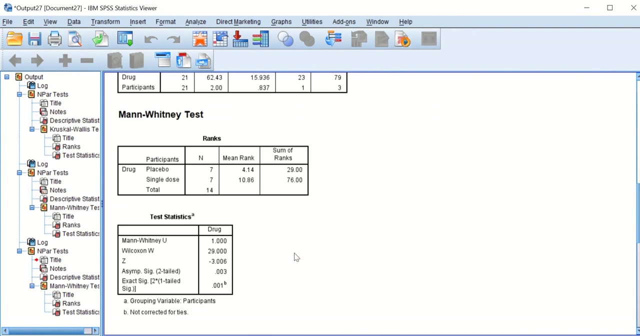 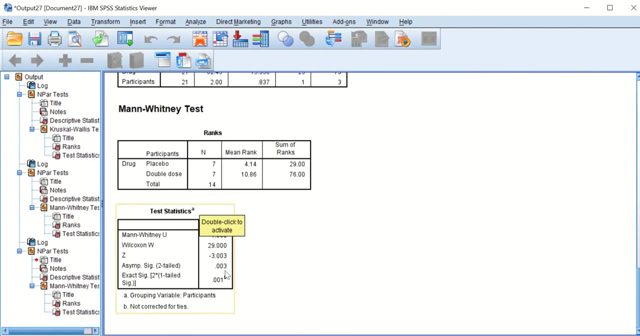 difference between between placebo and double dose. so we'll keep: group one is the placebo, group three is the double dose. click on OK, keep everything and click hit OK again. we can see that in this, in this test, in this test the value is again is also 0.1 between placebo and double dose of the drug. now if we again 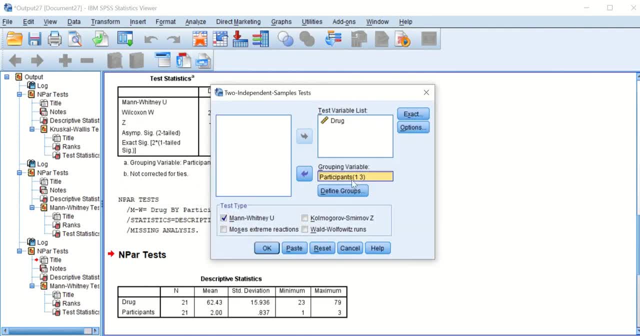 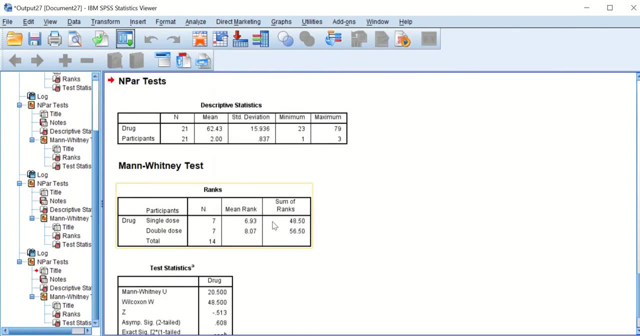 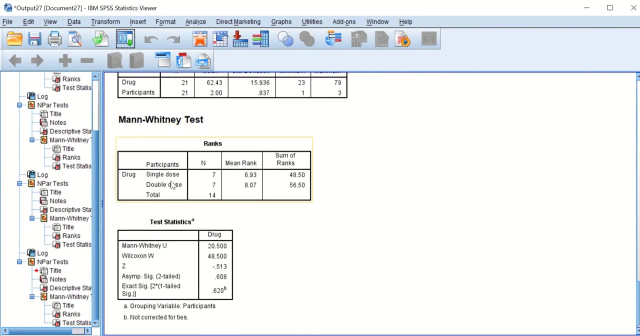 go back again and we do also the same test, but instead of comparing 1 to 3, we click on 2 to 3, click OK, keep everything the same. and again, man Whitney, you test has calculated difference, calculated the significant difference between single dose and double dose, and 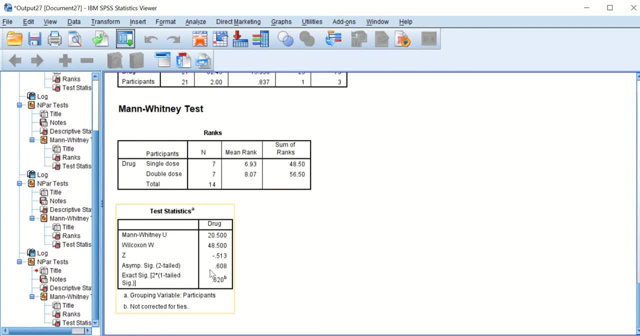 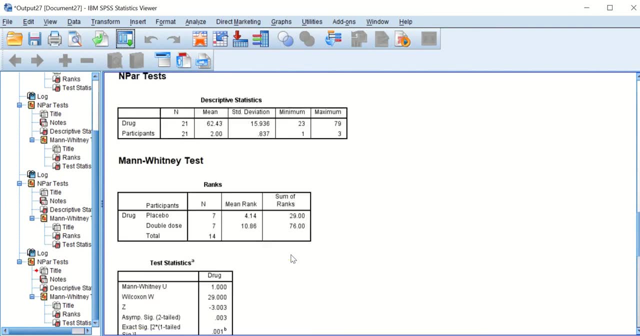 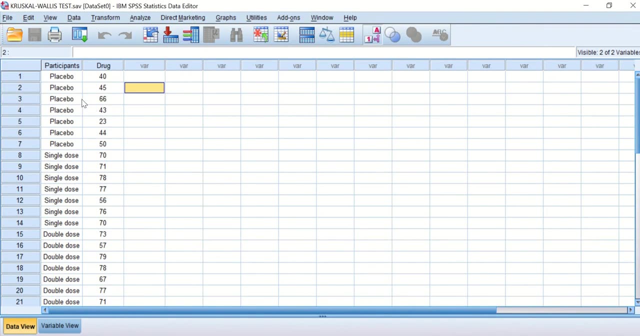 and, as you can see here, it is in fact no differences between the single dose and a double dose, as this p-value was 0.6. from this data, we can really, in a show that has shown that cares, Cal Wallace test that- tell you that there is a.